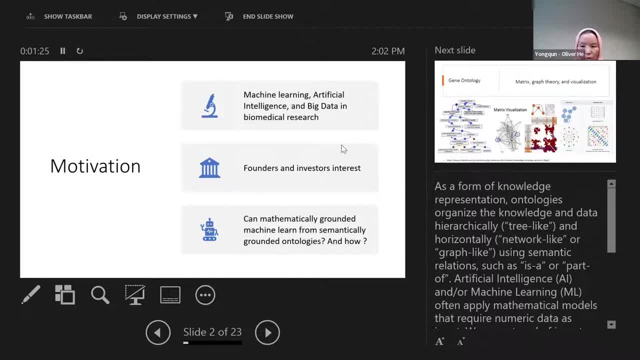 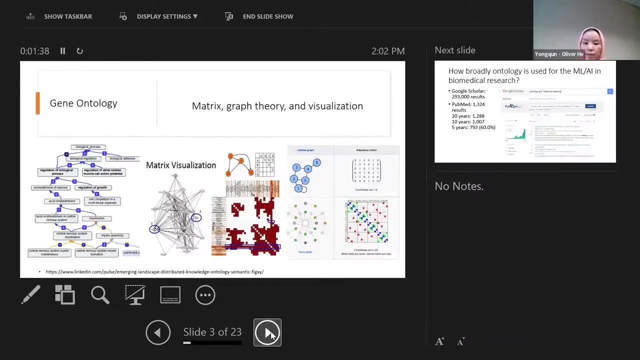 So then, I think the good way to start is just to look at what the literatures are out there, so we can have a landscape landscape analysis. It's not moving One sec. Okay, So we know that the ontologies are built with semantic simulations, but then all those graph theories and the data metrics are transforming the whole ontology into numeric input to the machine learning. 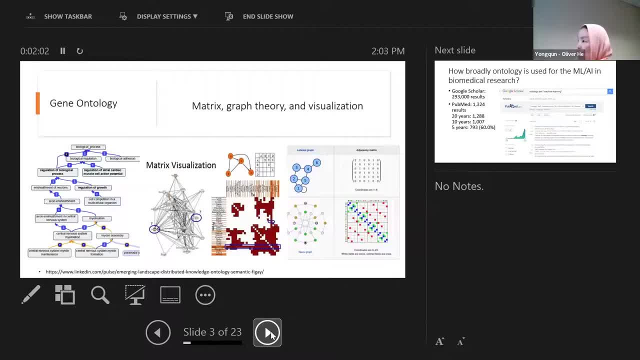 methods, But then how they do it and who is doing that- exactly the question that Rob was asking in the beginning. I'm interested in knowing that question too, because then we build a community, then we can have better result. All right, 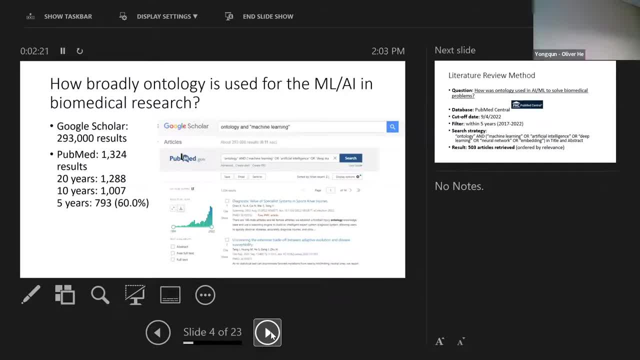 So then I started to look at Google Scholar. Oh my god, 2000, almost 3,000 times papers. And then I said, okay, I'm looking at the biomedical study, So I go to PubMed. It's good. I only find and I use better keywords. So I use ontology, machine learning, artificial intelligence, deep learning and the neural network. 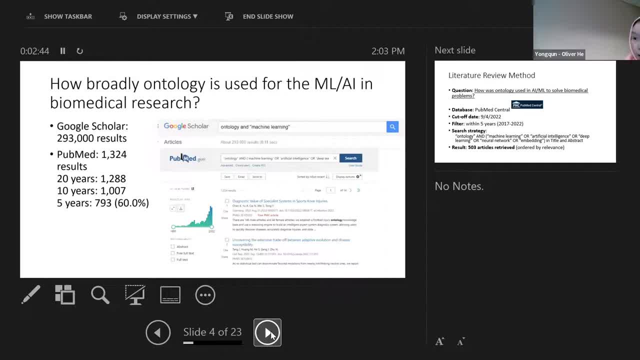 And I found 1,300.. And then I- but I just want to do a very quick overview- So I I did some filtering and I found the last five years composed 60% of paper out there, So I decided to use five years. 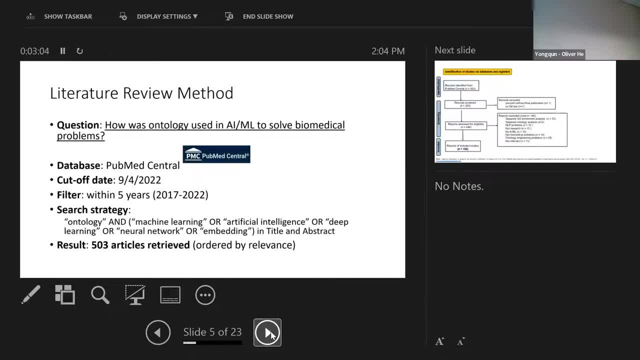 And eventually I went to the PubMed Central. Why is that? Because I can quickly look at the full text, I can look at their methodology and I can look at the technical details to determine if this paper is fitting to my question of how was ontology used in AI and machine learning to solve biomedical questions. 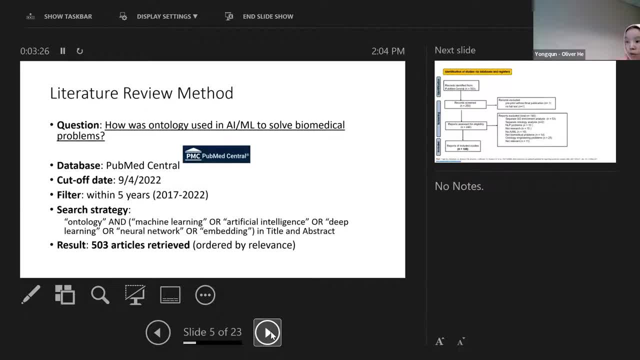 So I I- the cutoff date is the 4th of September- Filter: five years Search strategy, as I said, but I later on add embedding, because I see a lot of papers are talking about embedding. So by doing this I ended up. 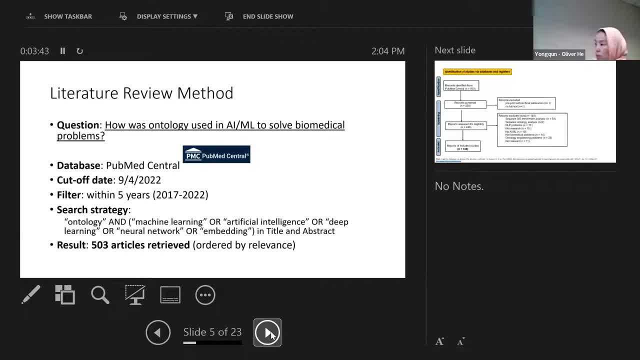 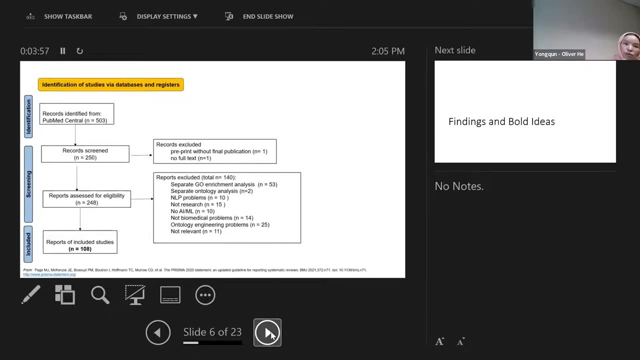 with 503 articles And note that the PubMed Central they are ordering the papers by relevance, So I screened 250 papers by relevance. So I think it's a very good representation of the 500 papers out there. And then there are some papers doesn't have a full text or preprint that I excluded. 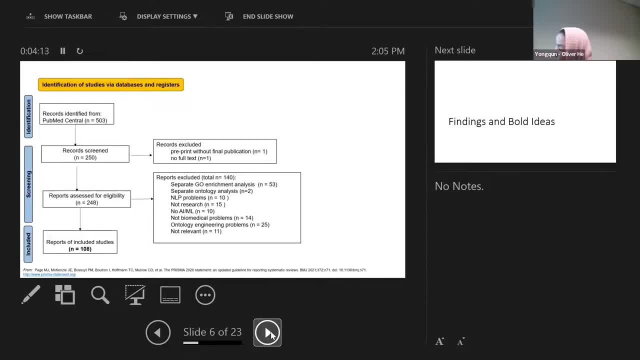 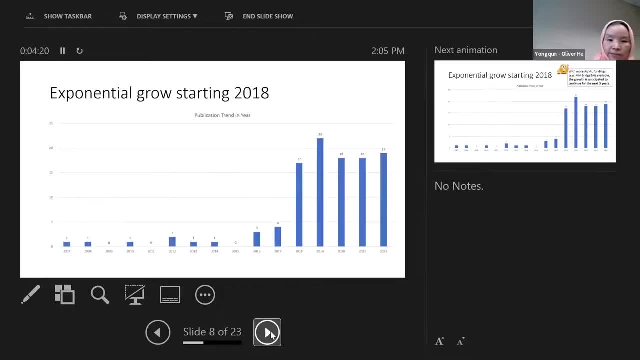 And then I did some eligibility screening So I ended up to have 108 paper to look. So the findings- The findings that I found after 2018, we see exponential growth there And I think this result is a little biased because suddenly I remember I just filtered five years data, right? So 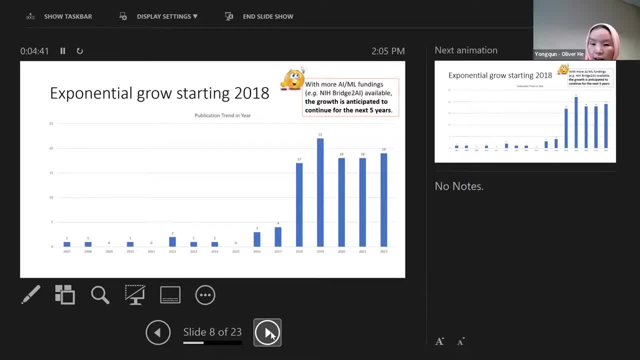 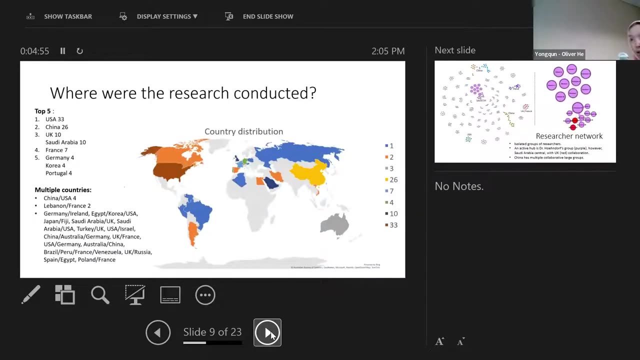 but still it's a big growth And since we are putting a lot of money, funds in the air And now I'm thinking that we will have more in the next five or even 10 years, So and then I look at who and where are those researchers are conducted, So it's very interesting to look at this map. 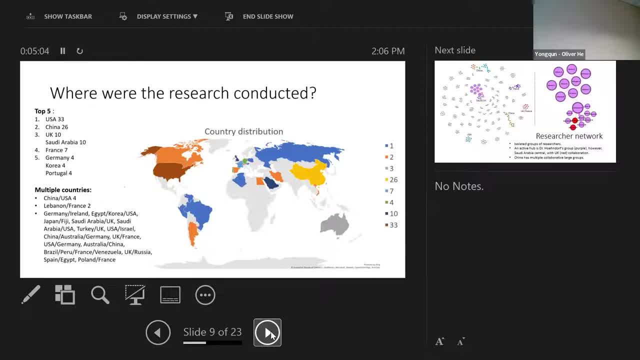 USA is the top one published country, 33 papers, And the second is China, 26.. And then in Saudi Arabia and UK, 10 by each, And then some countries in Europe, and then Korea has four papers, And there are also some. I want to see the how the countries collaborate with each other. Turns out that the China and the US combination on the top one, And then Lebanon and France. 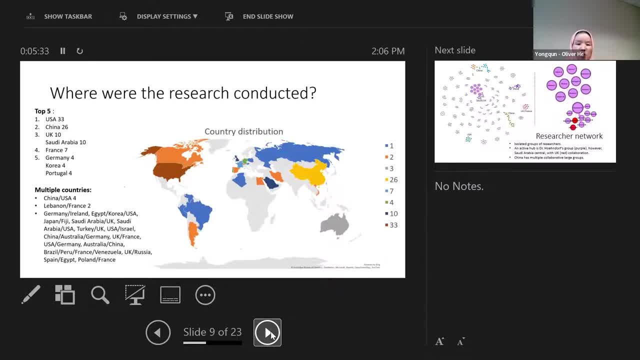 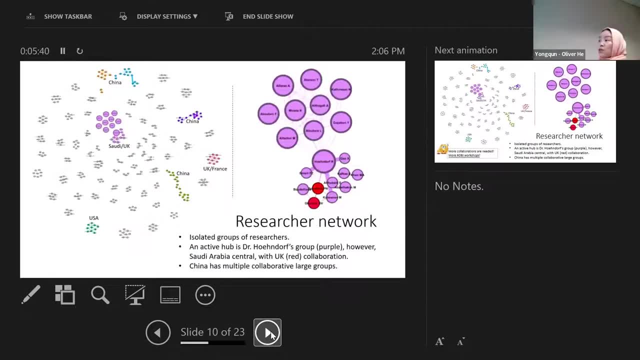 Saudi and the UK only had one paper, which is surprised, But maybe I so I will talk about my mutations towards the end. I missed a lot of papers for sure, And I also did a researcher's network, So what I found is also very interesting: A lot of- I see a lot- of- isolated researchers, right. 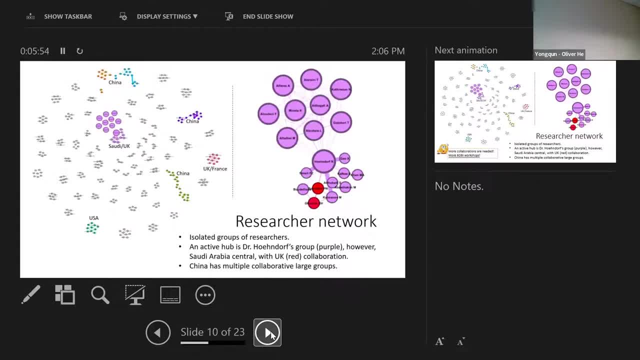 And then I found that Dr Honolulu, he is a hub for this whole research area at least, And then he composed two red dots here from UK- This one is another, our co-owner, Of course, co-organizer for this workshop, And China, because China has. 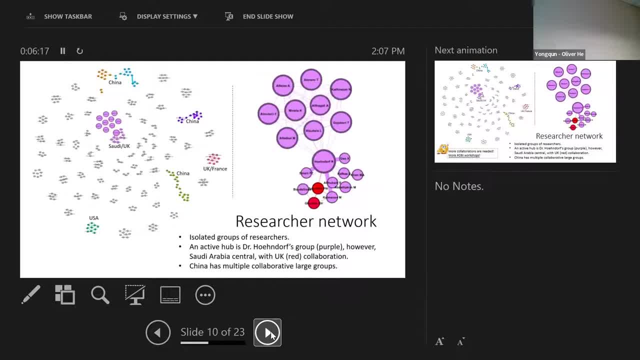 a lot of papers, So they actually formed a couple of in-China collaborations means the authors participate in multiple papers- at least two. That's why we form different kind of community there. So the conclusion here is that we need more collaboration and we need more Roving Workshop. 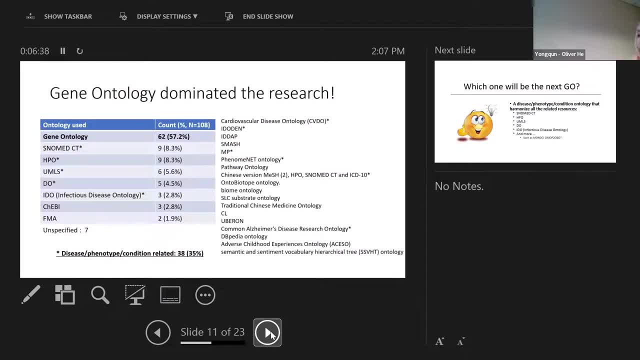 That's for sure, And also look at how which ontology I used the most. So I'm surprisingly, is not surprised that gene ontology composed 57% of the all the papers out there, That the 108 papers I screened And then next will be. really, they are not comparable to gene ontology at all. 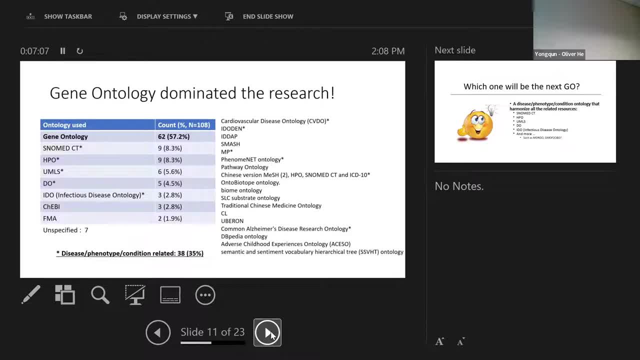 The Snowbank CT, HPO, UMS, DO. But on the right side of the screen are all those ontologies. really only appeared once, But if you are looking at, take a good look. I put a mark there. Those are disease or phenotype or condition related ontologies. 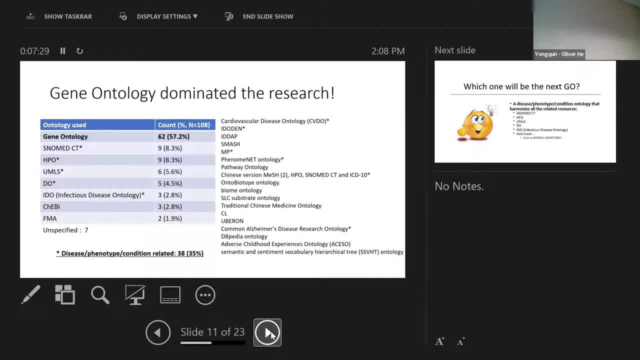 So if you add them together, they are composed 35% of the papers, So they are number two. Number two is about disease phenotypes and conditions. So and then I think, okay, so which one will be the next deal? 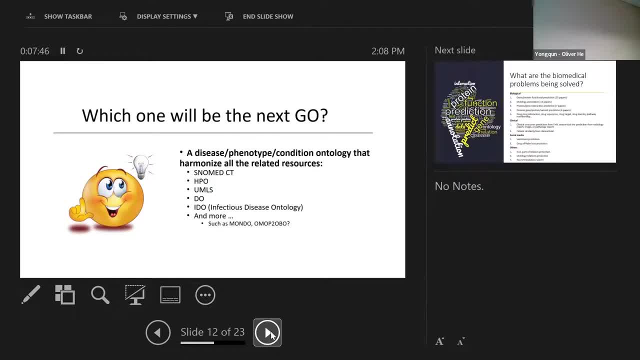 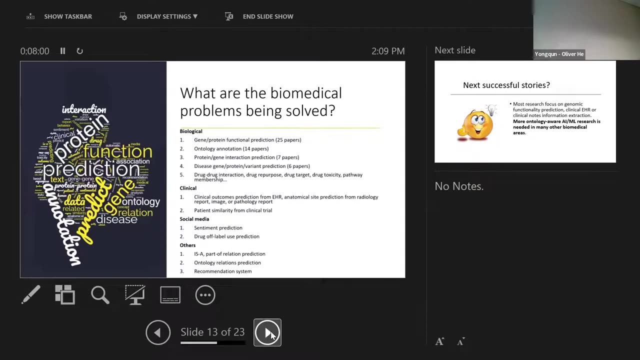 I think the next one will be a disease, phenotype condition ontology, that harmonize all those things, But I might be wrong. And I also looked at what questions the researchers are asking when they write a paper And I put them into four categories. But from this word cloud you can see a lot of papers are on gene or protein functional predictions. 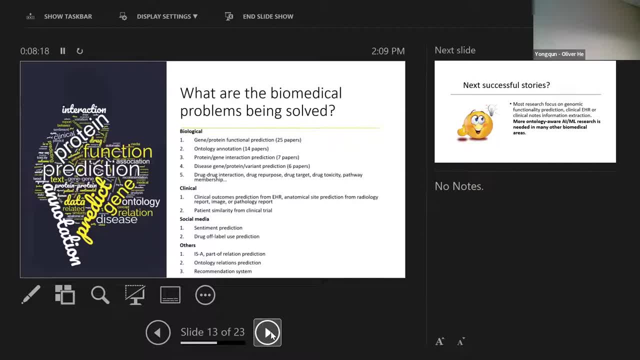 That's, there are a lot of people out there And then also a lot of papers using machine learning, artificial AI, ML- for the ontology annotation- Ontology- I'm not talking about a broad ontology- and cell ontology and all other conditional ontologies as well. 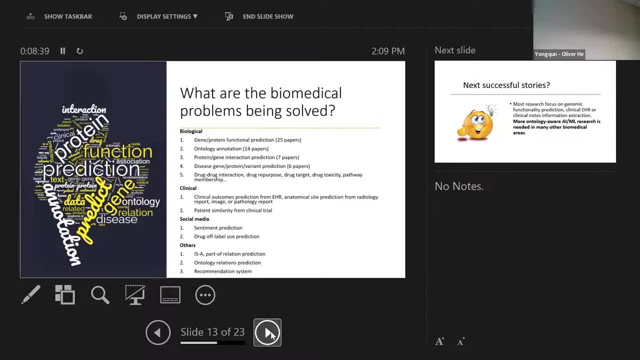 And then papers predicting gene-protein interactions and the disease specific genes, proteins or variant predictions are. And then you have drug related papers: drug-drug interaction, drug-repurposing- we just heard one Drug target, drug toxicity and then prediction of the pathway membership. 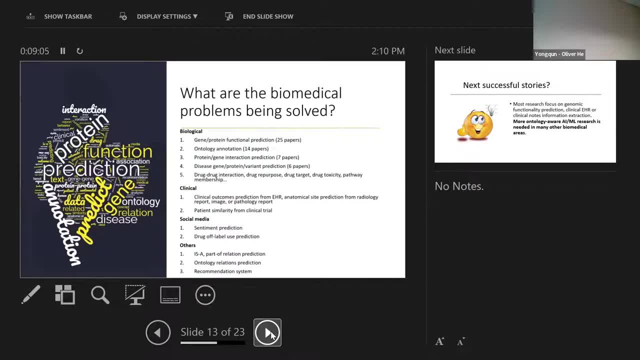 Then you go to clinical. It's very limited Clinical. mostly the papers are very limited. There are clinical outcomes, prediction from the EHR And there are a few papers too, Trying to predict the anatomic site, predict from the radiological report image or pathologic report. 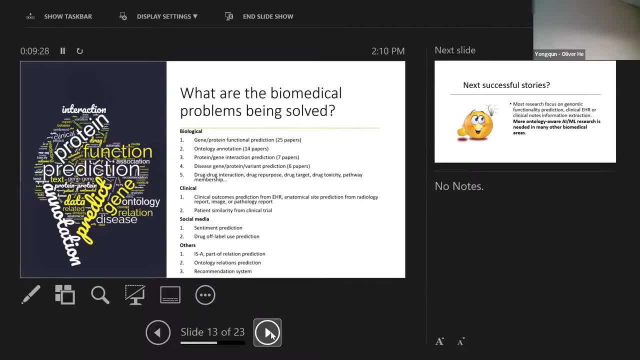 And then there is one paper looking at the patient similarity for clinical trial. So the third bucket is the social media. using those methodologies for social media And a couple of papers using it to predict the sentiment. One paper very interesting, using Tweed to predict drug off-label use. 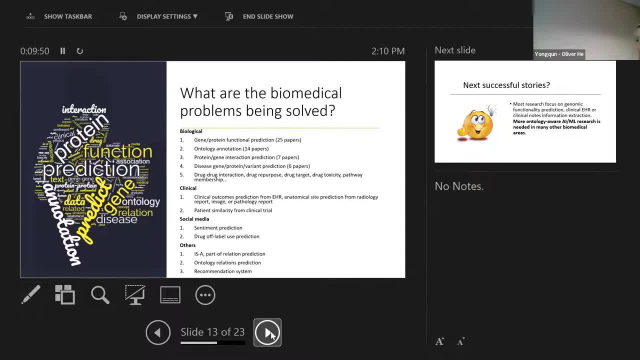 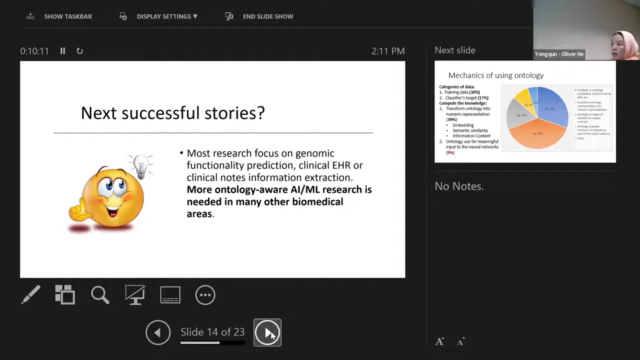 I think it's a very nice paper there, And then others will have some predicting the hierarchical relations in the ontology or part of the relation, Or just in general ontology, relation prediction and their recommendation systems using those methods, methods and ontology. Okay, so we know that in the biomedical field we have a lot of questions. 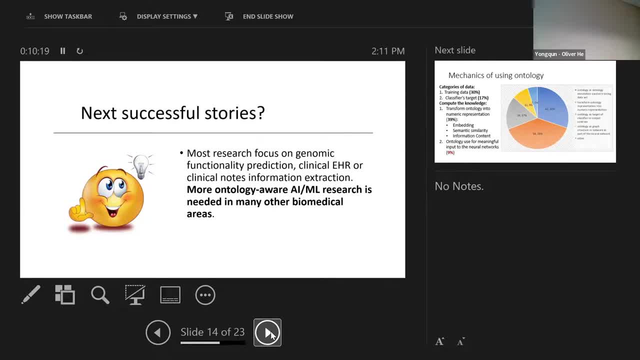 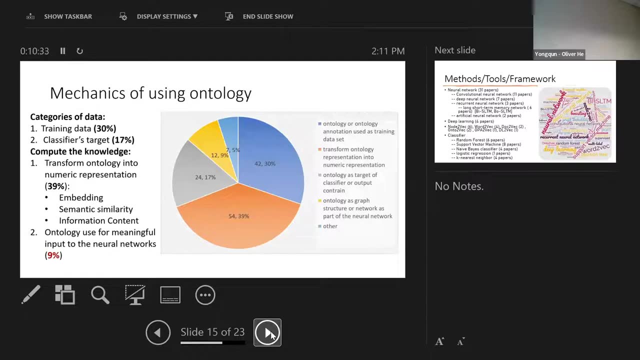 so I think we really need to get those methods to apply to more broadly many other biomedical areas That we need community help. So then I look at: okay, what are the ways people are using ontology for using for this methodology, right the mechanics. So one is the big category is use data. 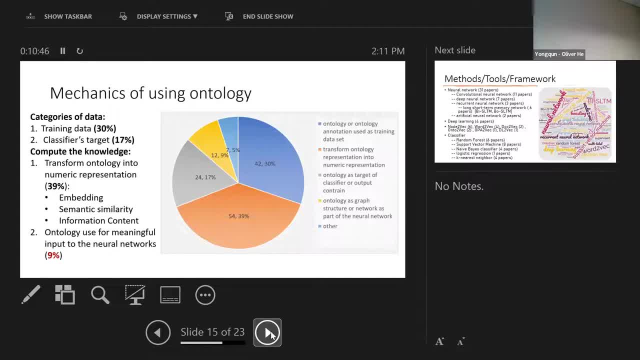 for the category use data as a training data set or use ontology as a classifier target. And then another bucket is: I use the ontology as a part of the machine learning method so that I can compute those knowledge. So I found 39 percent. 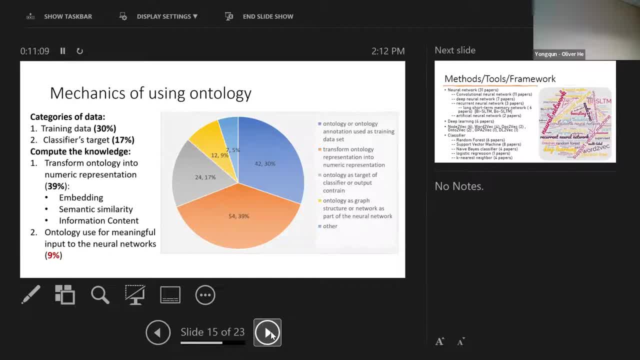 that are using embedding semantic similarity or information content. So this is exactly how you are transforming all those words and the relations into a numerical data matrix. They use all kinds of ways to try to get a numeric presentation for what ontology is coded in. So I see a lot of 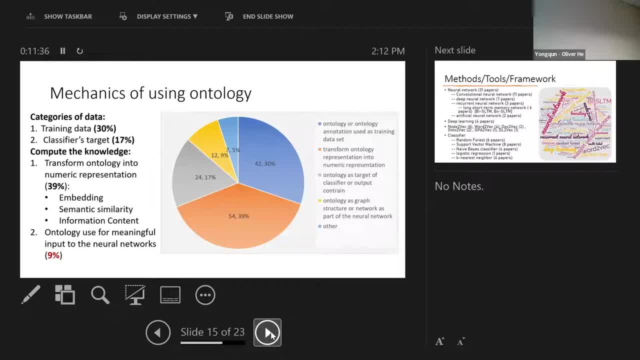 fantastic papers out there. However, we are really looking. we're really lacking of the those ontology use for meaningful input into the neural networks. There are some papers using the ontology and ontology annotated data form: the network as the layer of the neural network, but not too much, not too many. So we're still lacking. 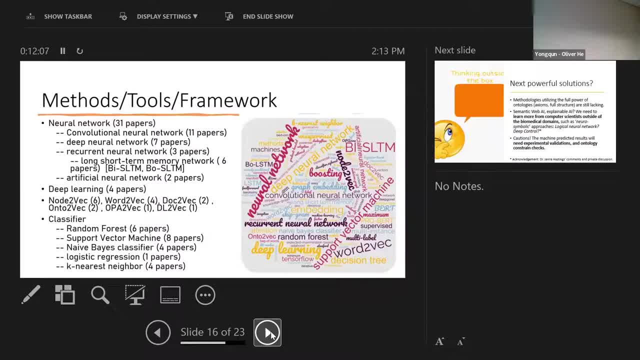 And then I also at what are the popular neural networks or deep learning, or all methods are there. So the neural network is the top one, probably related with my search word, but the convolutional neural network has a lot of paper using that and then any other neural network, And today I learned about 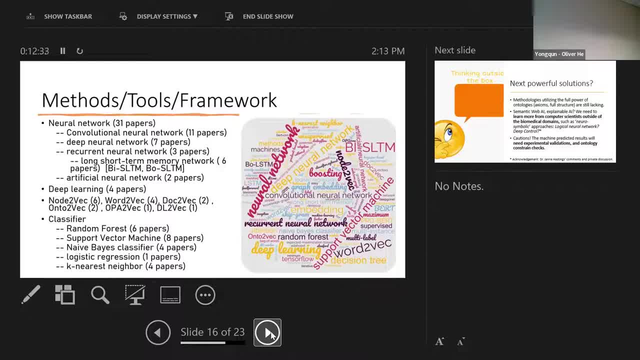 graph neural network. so there are a lot of neural networks out there. And then we have some papers on deep learning. We have a lot of papers on using vectors, transformation methods. so we have node2vec, word2vec, doc2vec, onto2vec, opa2vec, dl2vec, and I just noticed there is a add2vec. 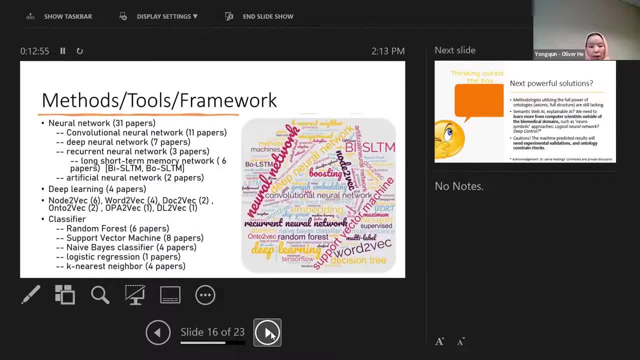 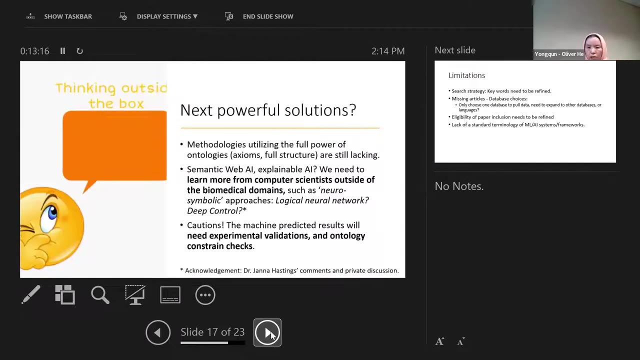 the previous talk. And then still people are still using the classifier, the traditional ones: Random forest, SVM, logistic, Bayer's, McKenna, Pay, KNN. So there are still people are still using it. Okay, so what we need here? as I said, we need more paper. 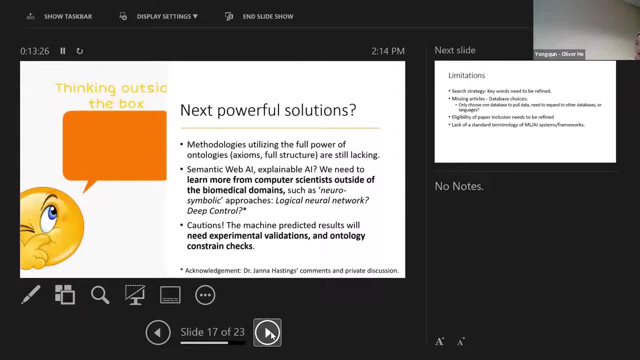 to think about how we utilize the full powers of ontologies in those high-end AI ML methods. So I saw out there there are semantic web AI, experimental AI, which are the possible solutions, and also learned that there is a neural symbolic approaches that can be possible solutions. I think we need to implement that. 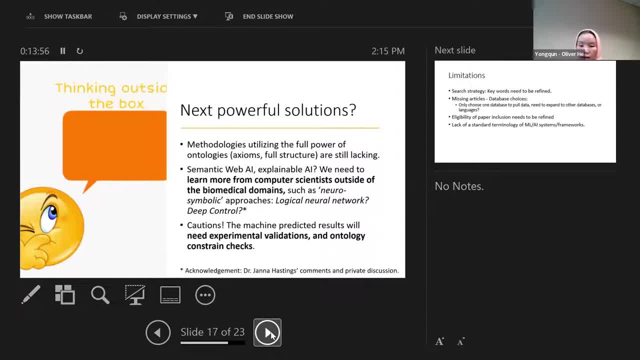 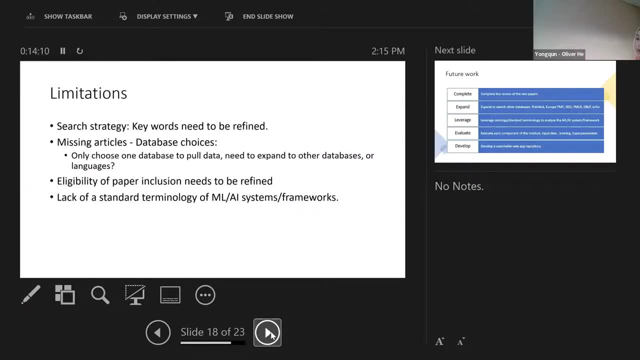 But I need to put a question there and I will talk more in my panelist discussion- that those predictions, we really need experimental validations and the ontology constraint checks, All right, so the limitation for this work- and I'm still, it's an ongoing work, I'm still working- 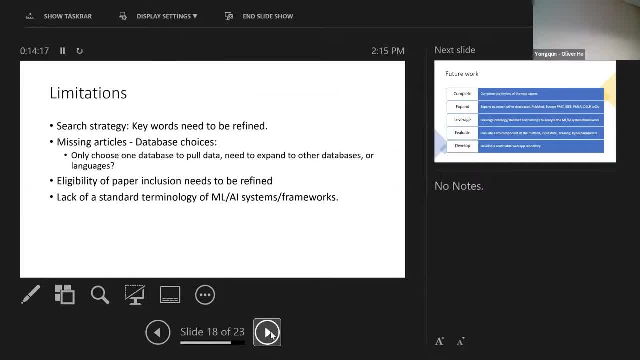 on. it is that the strategy, search strategy. we may need to refine the search strategy and also ontology, the database choice. I only choose one database. there are a lot more out there that I need to search And I might need to refine eligibility And there is a lack of standard terminology for those. 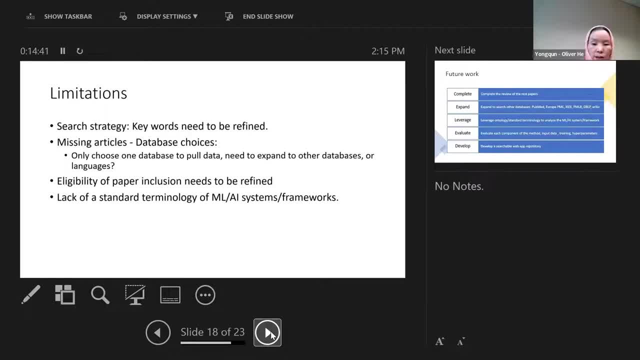 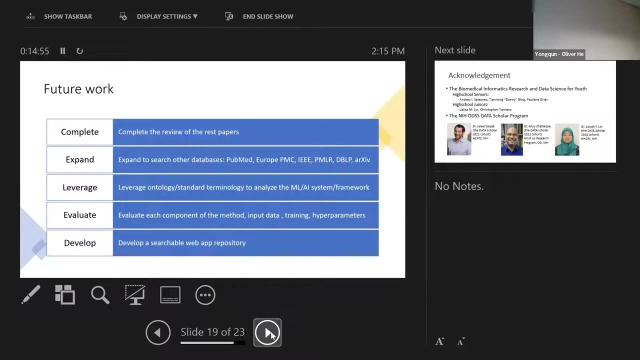 AI ML systems frameworks. Fortunately, I found one paper who is developing this kind of standard terminology so I can use it for my future work. So my future work, I will spend the database. besides completing current work, I expand to other databases. 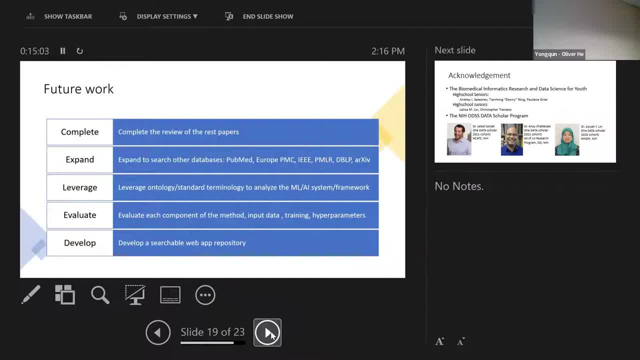 databases, especially the EURO-PMC, and some computer science databases like IEEE, BDRP, PMLR and also some preprint database. Then, as I said, I use the terminology to really put it in a standard form, so I can analyze better And then I will do more, deeper dive. 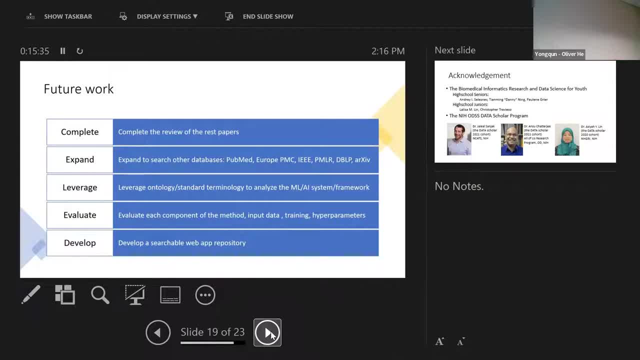 into looking at how they use the input data, what methods they're, what hyper parameters they're using and what training data they're using and what performance evaluation parameters they're using. So then I can maybe view the database website. Everybody can search All. 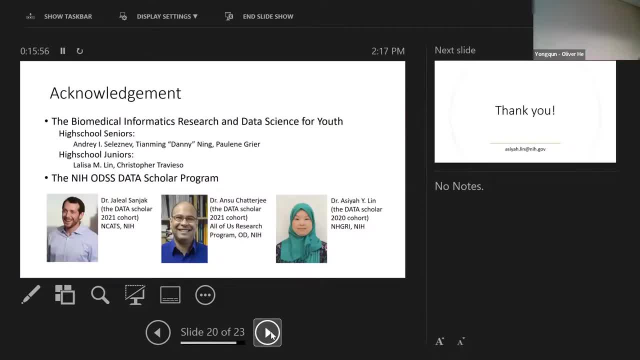 right, I washed my hands. This work is run by some of my high schoolers. I have a volunteer group by medical informatics, research and data science, So the high schoolers have helped me to prepare the data, and I also have two other data scholars to join me. Oh, by the 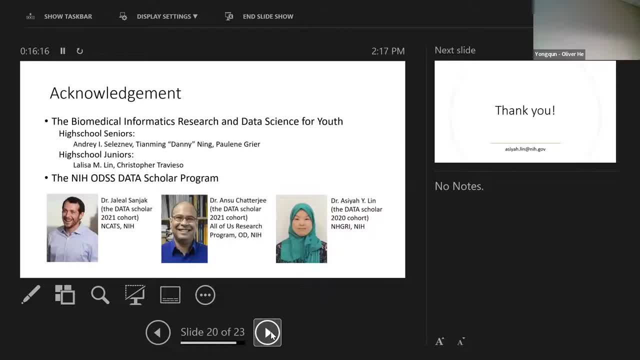 way. so the Data Scholar is a special program from NIH. Their full name of that is Data and Technology Advancement- Before make real a one year or two year program to get some senior technical people to help NIH for a lot of data science heavy projects. so I have two other data scholars join me with that. I thank you. 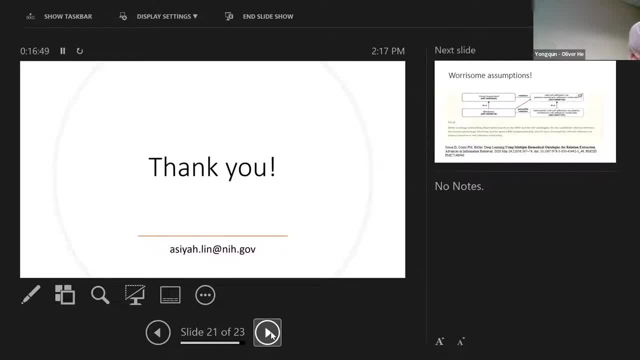 time for questions or comments. so a lot of your graphs include the quantity of data. though, when looking at the quality over year over year, do you think something like an age score would help determine age scores to help determine quality, or how would you look for quality? oh, I'm not familiar with each score. citation numbers: oh okay, I didn't. yeah, I didn't use. 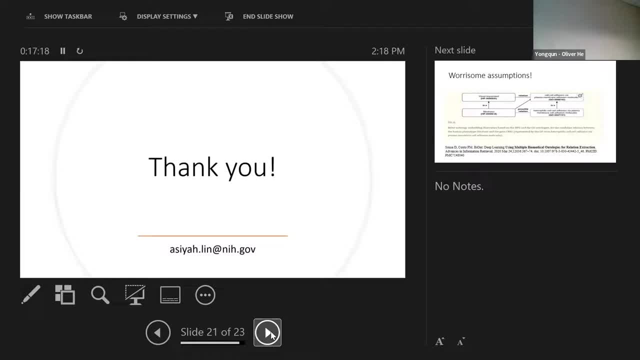 incorporating that, because I just want to have very quick like view of what is happening, right. but I should add, yeah, thank you so much. did you? did you uh, work with or consult with a librarian, um, with your search strategy at all? no, I did a lot of literature reviews at FDA, so and uh, yeah, okay, 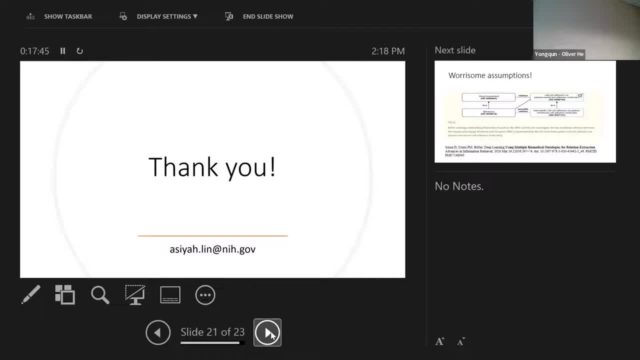 I've used them in the past and when it comes to coming up with they have a very big one, yes, but my, my point is: I want to search. very broad way of searching. yeah, yeah, I forgot to repeat the question to the oh yes, yeah, the first question was: 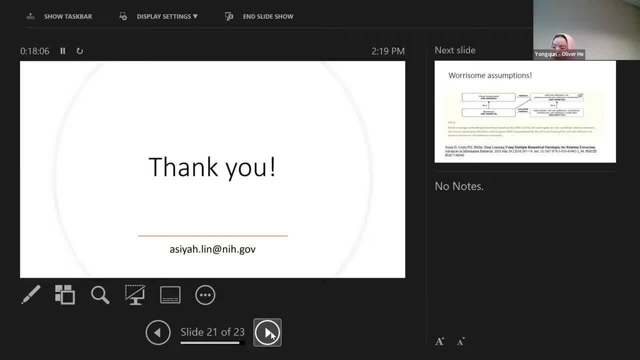 about. do I use the h score like the citation, including citation for the tour to, for the paper's quality? I didn't and I didn't know h score, so I will use it for my future work. and the second one was asking: do I ask a librarian help? I said no because I did a lot of. 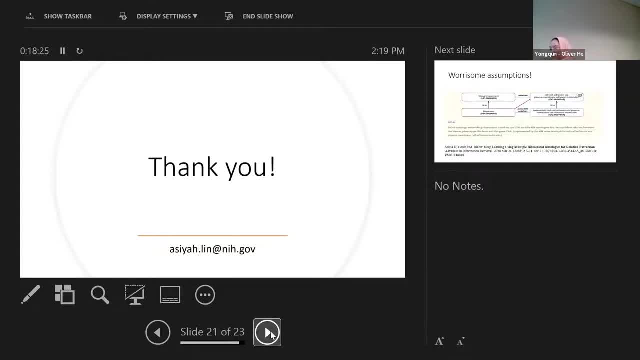 literature review. yeah, thanks for sharing that. I think you're right. the research you did can help answer some of the initial questions. I think you can. I would like to suggest that you multiply your impact by using uh when you say you found that these kinds of uh activities. 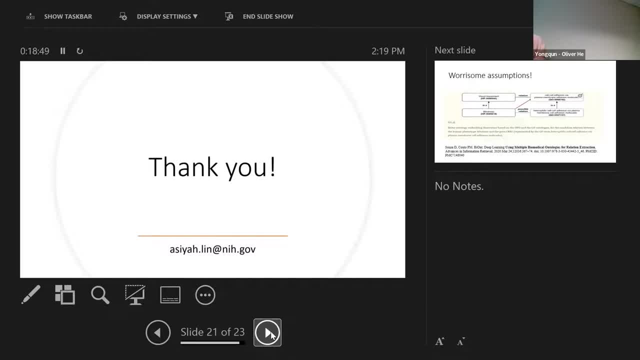 were performed, such as classifying within ontology or using ontology. as I've been aware that you're in ontology, you could actually classify those outcomes according to classes in ontology, like the artificial intelligence ontology. yes, and you can do the same thing for when you describe a different uh, which ontologies, or what's frequently used in ontology, AI, yes, uh, you could try to form. 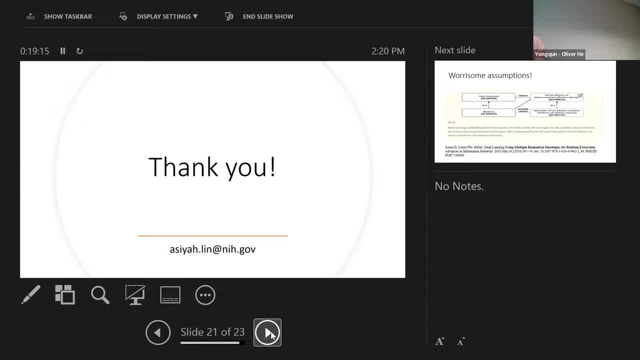 an ontology of ontologies and say what? what are the characteristics that have made SNOMED more useful than than the plant ontology? something like that, And you can even one of the questions could be: are the ontologies that are most useful for machine learning? are they more A-box rich? 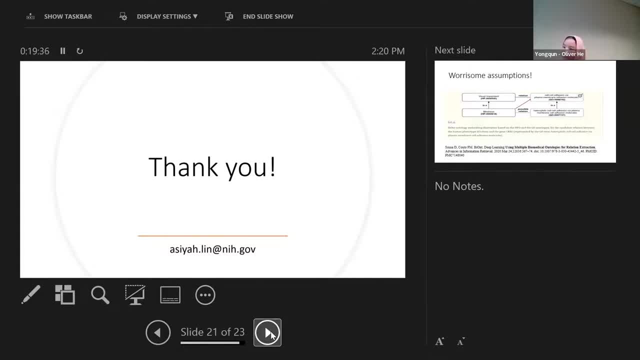 or are they more T-box rich? Because SNOMED has a good mix of both, whereas something like. so. if you speak purely in terms of the Go ontology not going to include classification, gene ontology is mostly T-box Gene ontology. I see most of them using 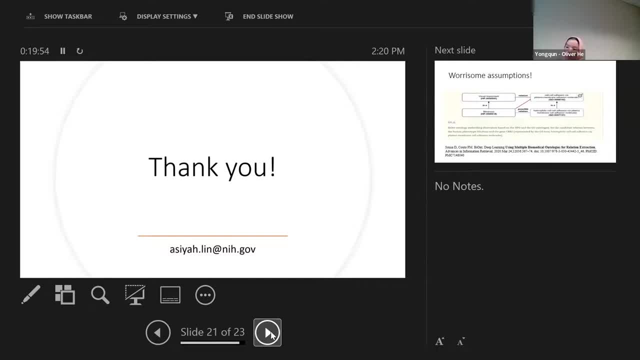 the annotation of the gene ontology Couple of. yeah, those are great questions, So I repeat the question. He gave me a couple of very good suggestions. One is using artificial intelligence ontology to classify my result. that was in my future plan. I agree with you. 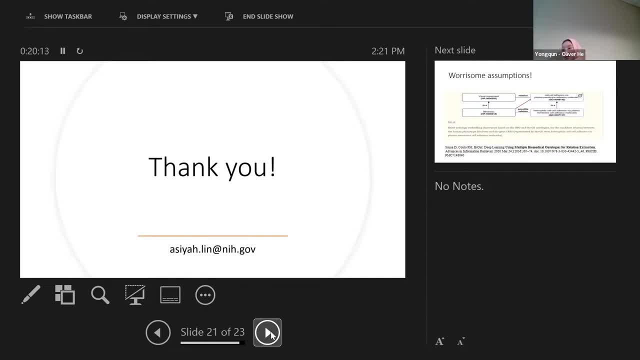 The second. what is the second one? It's simple, the artificial intelligence. ontology to classify, Oh, To classify the activities that we use and also things. could you make an ontological model of which ontologies are most useful and what is the distinction between them? 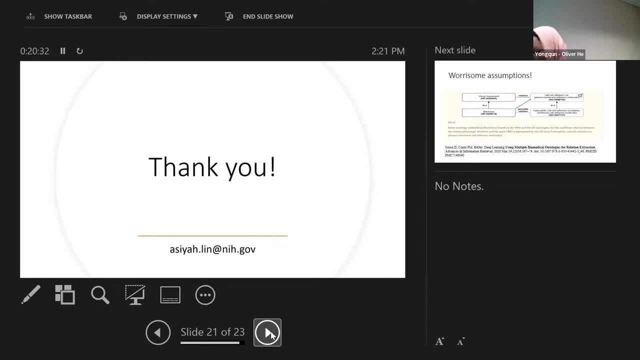 Right. and the second one he suggested me to it's Mark. he suggested me to develop ontology of ontology and to find out which are the most popular ontology and find out if the ontology is being used as a T-box or A-box. So I kind of I have seen that gene ontology. 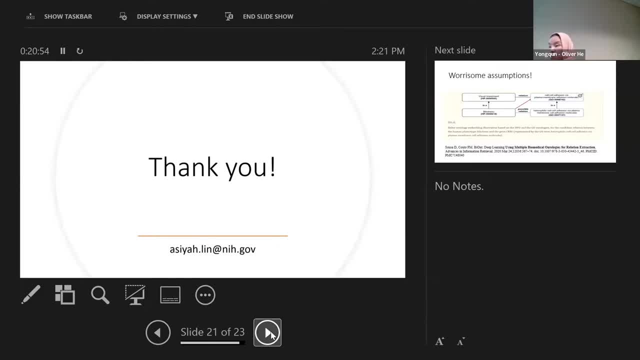 has been mostly using gene ontology annotation And I have to. I noticed this When I searched gene ontology in the PubMed I screen. I excluded a lot of papers because a lot of biomedical bioinformatics paper. they would do a prediction. 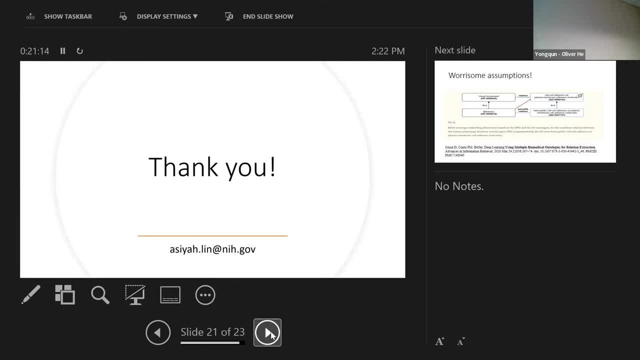 They would do a like expression gene analysis and then they coupled with the gene gene ontology enrichment. So that is a big thing I have to filter out. I filled out a lot of papers on that. So if you search gene ontology you got a lot of things that you have to get rid of. 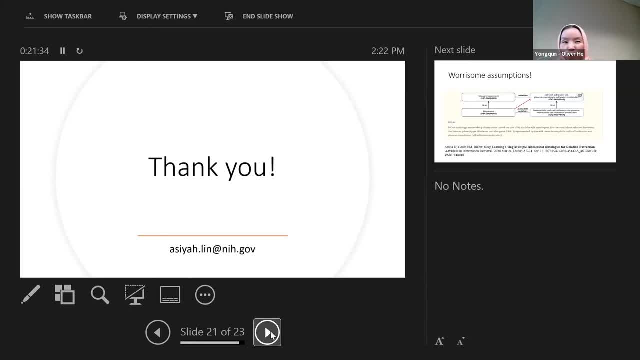 for my purpose. Well, thank you so much for all your suggestions. I actually I need to recruit people to work for this.